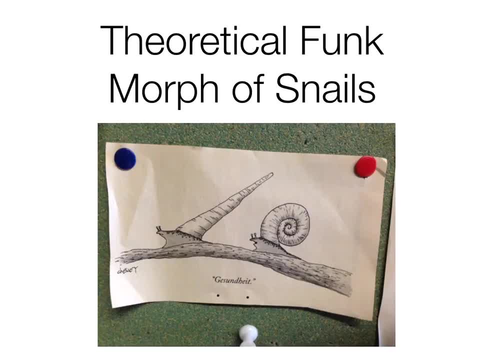 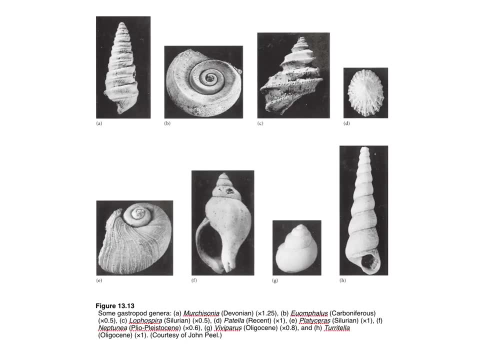 my favorite New Yorker snail cartoon for your enjoyment. So snails are gastropods, they're within the phylum Maleska and they take lots of different forms. So here is just a figure from your textbook showing some of the different morphologies that snails take. 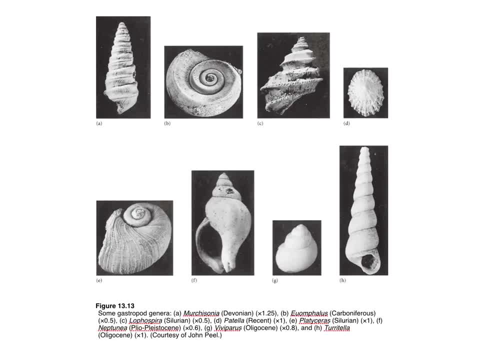 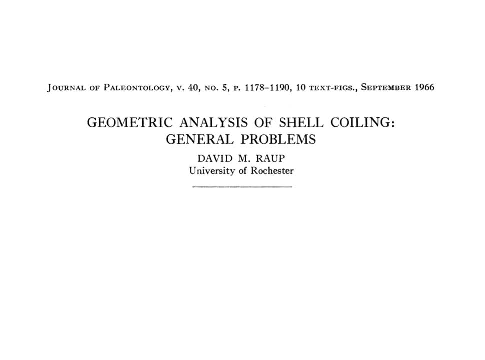 So the question is: why do snails take all of these different shapes? And the person that asked this question was a paleontologist named Dave Raupp. Raupp was a really influential paleontologist who was very quantitative and he was one of the first paleontologists. 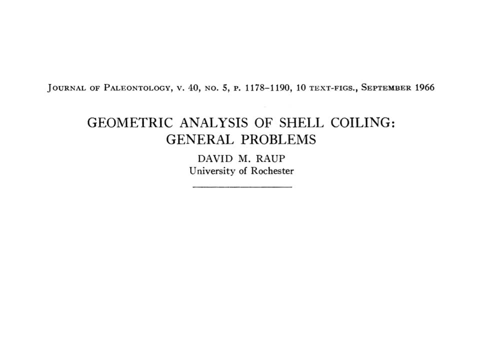 to really apply a lot of quantitative skills and tools to the fossil record, both in terms of diversity analyses, which we'll talk about in the next lecture, but also in terms of the geometry of different organisms. So this is his geometric analysis of shell coiling. 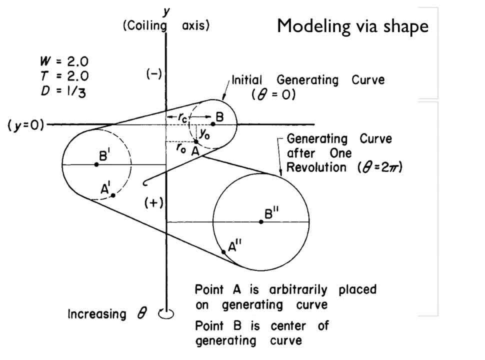 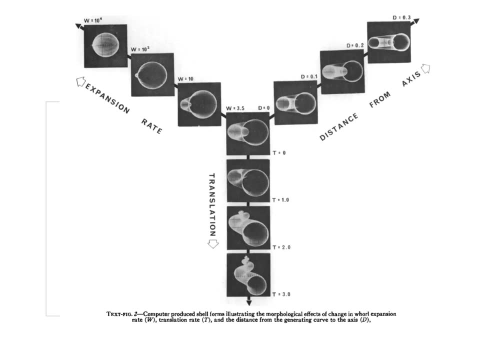 So what he did is he basically made a model of how a shell coils And he came up with a number of different variables. He described all the different ways in which you could make a shell And I'll just go over those here. So the different variables are in the top right, distance from axis, So you 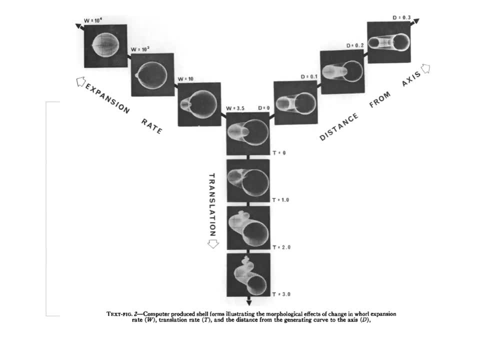 can think of this as sort of like a loose coil or a tight coil. On the left corner is expansion rate, which is how much the diameter of the shell changes as it curls, And then down the middle is translation, which is whether or not the coiling of the shell goes up and down or 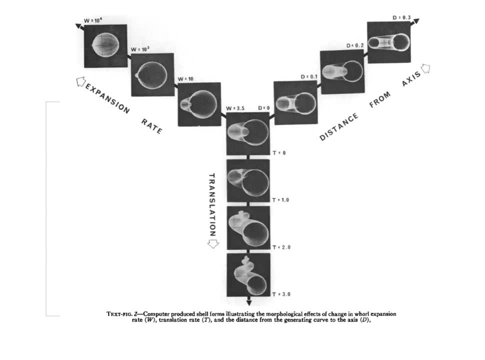 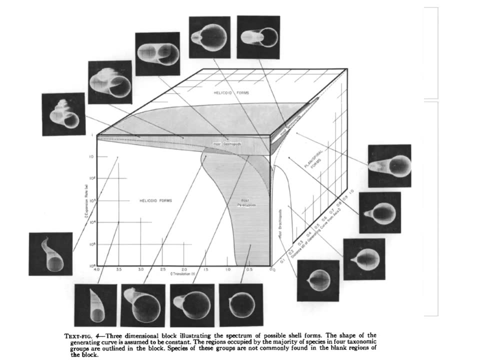 just stays in one plane, So it doesn't sort of become a high spired, or does it just coil in one single plane. And so what he did was he then made a theoretical morphospace using these three axes, And hopefully you can see this. I've also posted a PDF of the slides where you can look at them, probably in higher 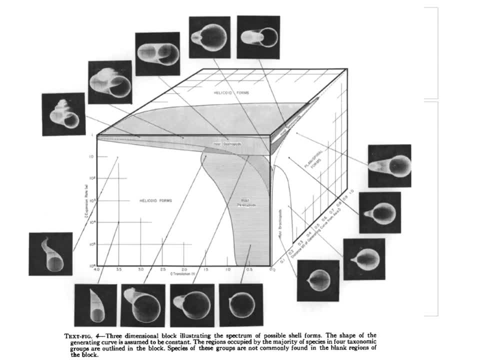 resolution. So what you can see is we've got our axes. So the axis on the bottom right is distance generating curve, On the bottom is the translation And then on the other side is expansion rate, And the shaded in areas are the only areas where we actually have 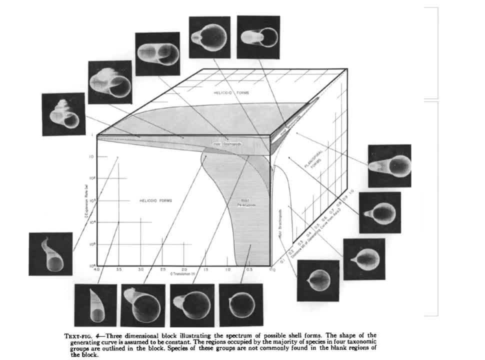 living or fossil specimens that represent those forms pretty much, which is pretty cool. So we can see that we've got, you know, different snail forms. We've got limpets in, like the right hand side, So limpets don't really have any coiling at all, So their distance. 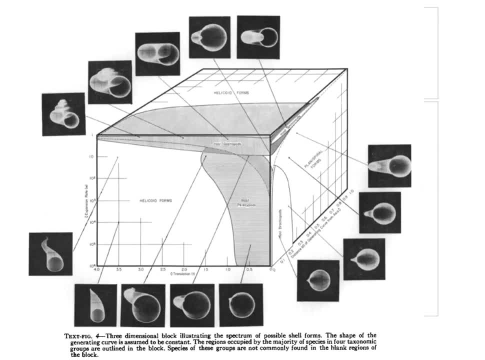 from generating curve is really small. We have different types of snails in that top gray area, depending on whether or not they they coil within a plane or out of a plane and depending on whether or not they're loosely coiled or tightly coiled. And then there's also some points that he's highlighted in here where we don't find organisms that make these shapes. 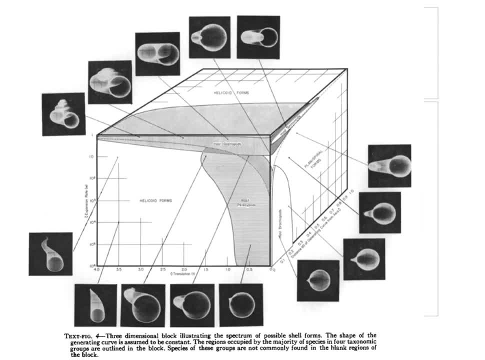 And so one example is: on the left hand side You see that sort of like elf hat looking like this one right here. So this one falls into a point right here and there are no living or fossil snails that have the shape. So you can think about why that might be. 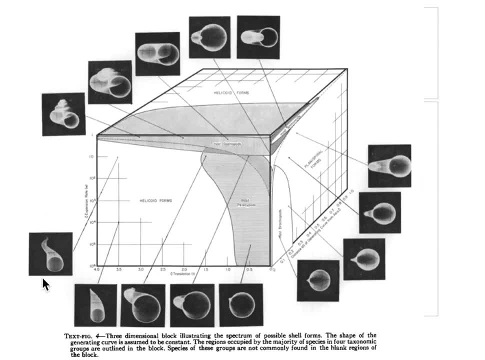 Right. Is it a structural thing? This doesn't look very robust. You'd look like you could sort of snap the tip right off of this thing, right? So it's perhaps evolutionarily not advantageous. Similarly, if we look over here at these really loosely coiled ones here, 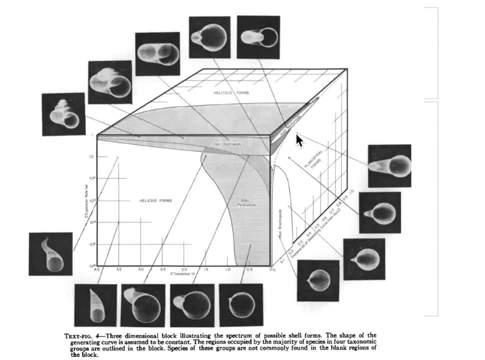 again. you can imagine that a very loosely coiled snail shell would be very easy for an animal like a crab to crush with its claws, And so the areas that we see filled in here and up here, which is the trapezoid. 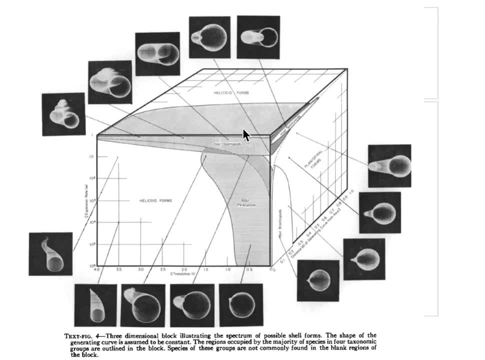 which is sort of our more normal snail shapes. you know, there's a ton of theoretical morpheus space in this cube that's not filled, And so by thinking about what is filled and what's not filled, we can think about the structure and function of a snail shell in a new way, which I think is pretty cool. 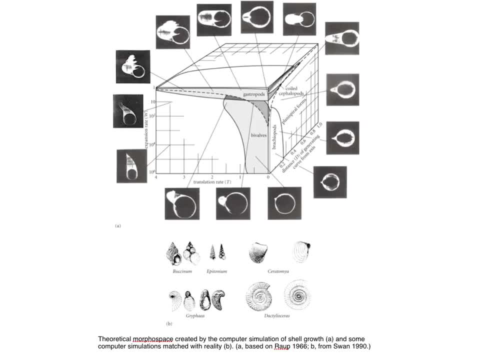 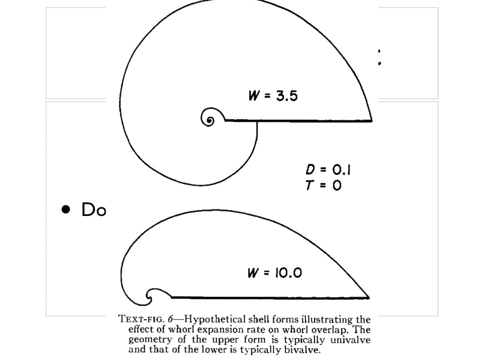 And here's just another diagram- I think this is from your textbook now- showing again basically the same thing: The actual species are not randomly distributed. There are constraints within the spectrum. This is basically the same thing. showing again whorl expansion rate and overlap so that like